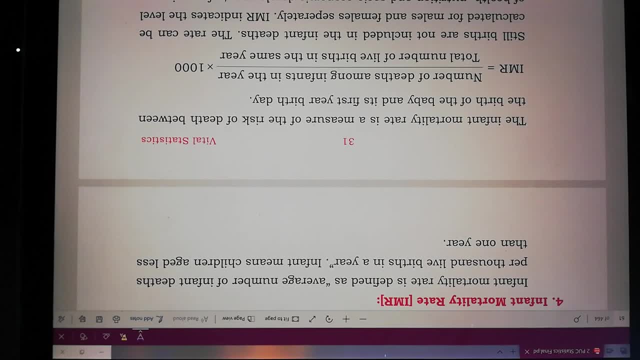 problem with some set of data that they give it to us, but it will be only of two marks. so that is the reason why let me take this opportunity right now to solve these problems. first, ready Ammar, NMR and MMR problems. so I am mark infant. 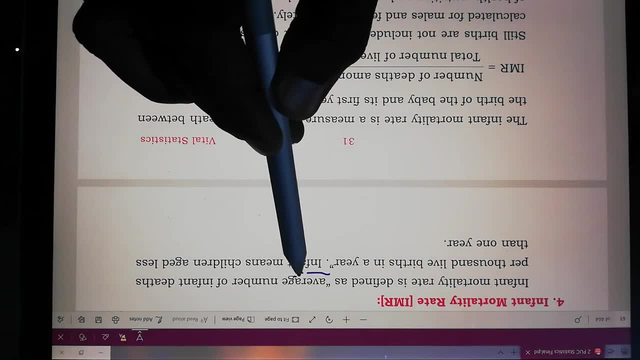 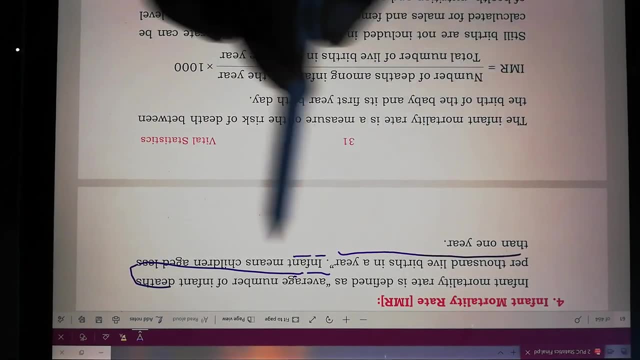 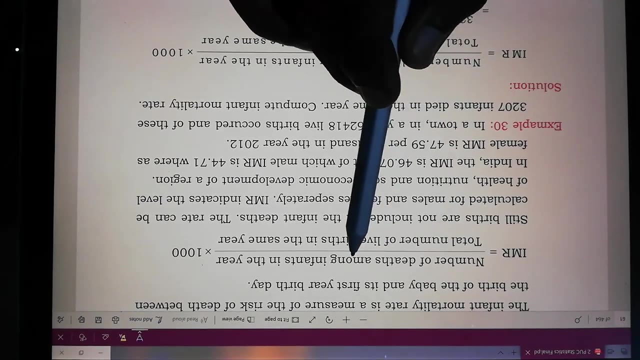 mortality rate. infant mortality rate is the average number of infant deaths per thousand life births in a year. what do you mean by infant? infant is a children aged less than 1 here, okay, the formula is given to us by this number of deaths among infants in a year. okay, I hope you are following number of 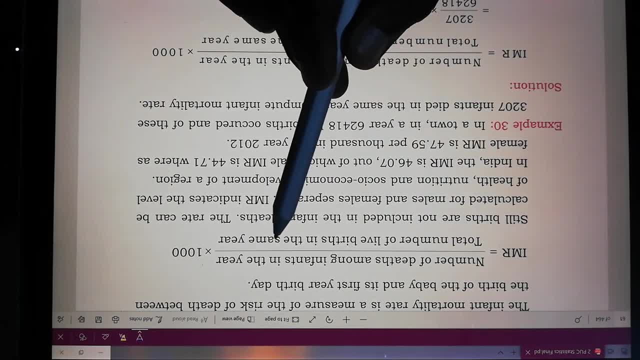 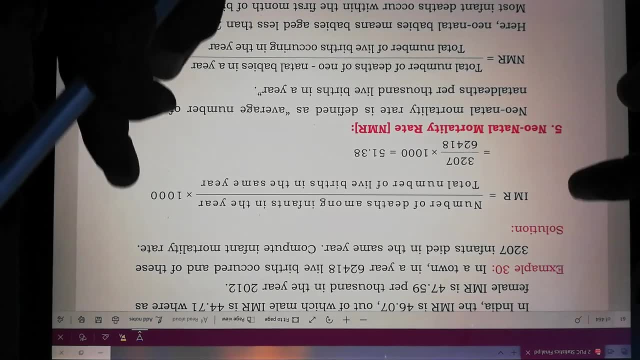 deaths are infants in a year divided by total number of live births in the same year in 2000. okay, so the calculation is very simple if you just take a simple formula that is given to us in the textbook: in a town in a year. you want me to expand it? 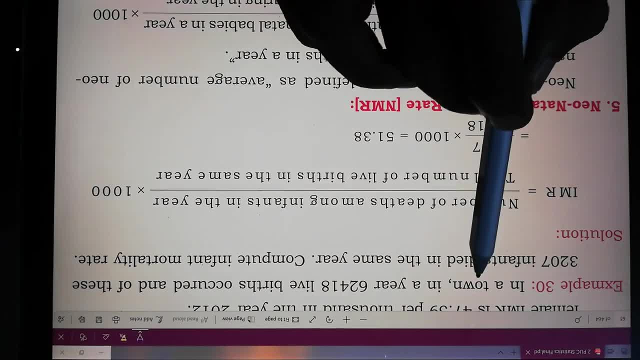 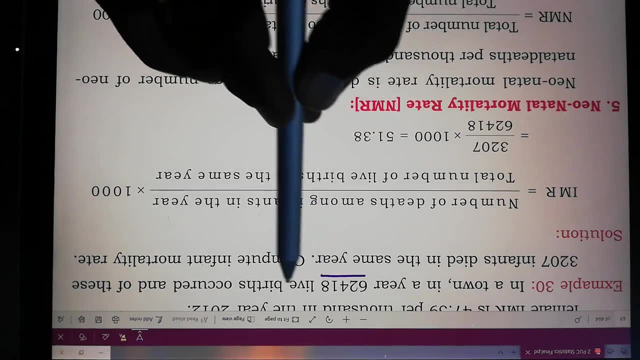 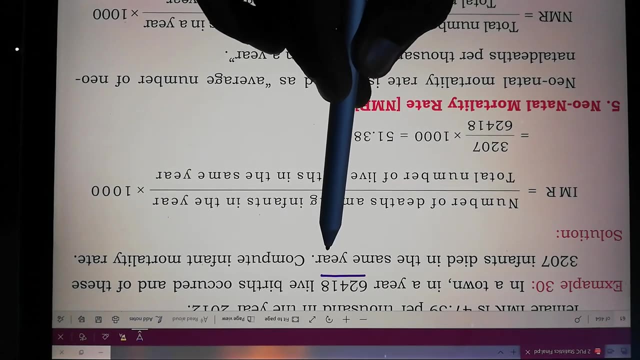 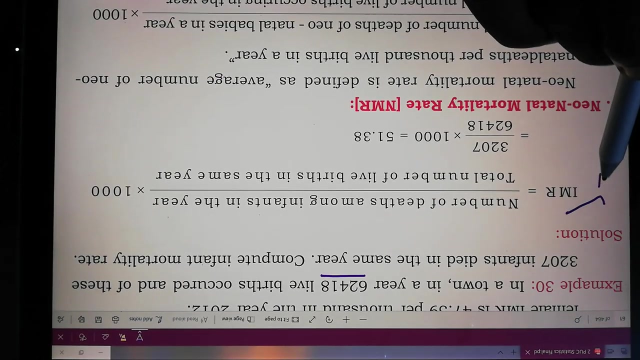 yes, you see it more clear. in a town, in a year, sixty two thousand four hundred and eighteen live births occurred. live births occurred and of these, three thousand two hundred and seven infants died in the same year. compute infant mortality rate, IMR. so first write the formula. students, this carries one mark. 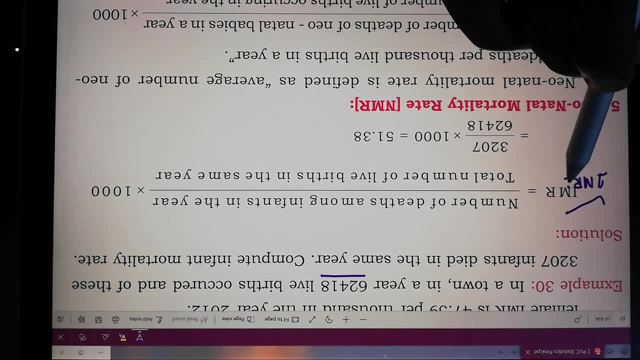 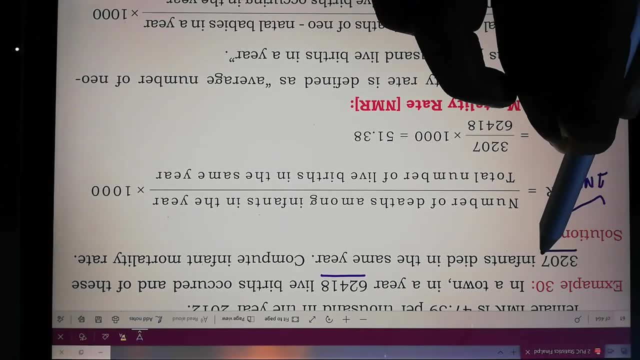 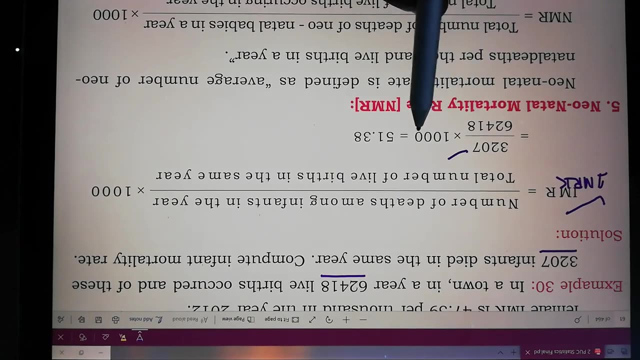 writing the formula carries one mark, okay, one mark. so after you write the formula, then put the values here. number of deaths is three, two zero, seven, okay, number. total number of live births is sixty two thousand four, eighteen, sixty two thousand four, eighteen into thousand. so you get fifty, one point, three, eight. 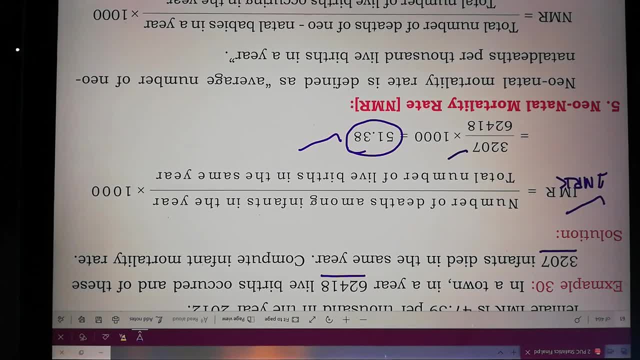 this is a simple problem. okay, IMR. so vice versa, students, they may ask you IMR, they may give. like you know, we have calculated CDR in the previous case. IMR, they give us, they may give us the live births and they ask us to find out. 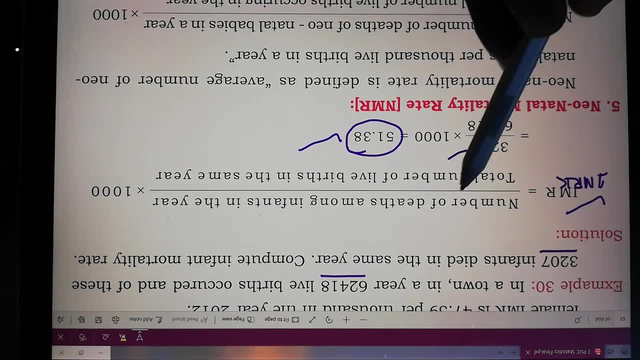 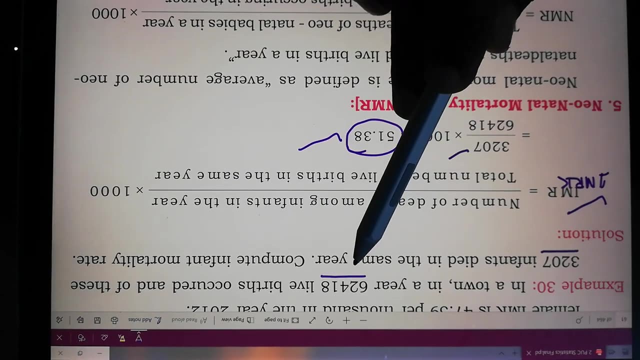 number of deaths among infants, or they give IMR. they give number of deaths. they ask us to find out number of live births. okay, it is quite simple. so you have to read the question carefully. what is given to us? based on that, write the formula. according to that formula. what data is given to us? fill in the data you. 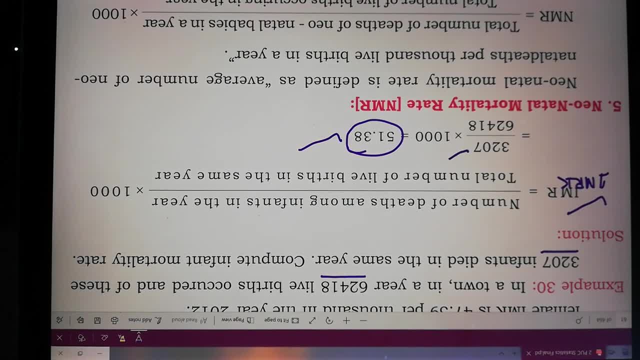 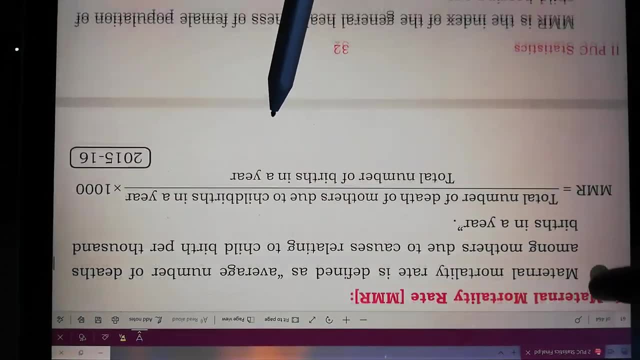 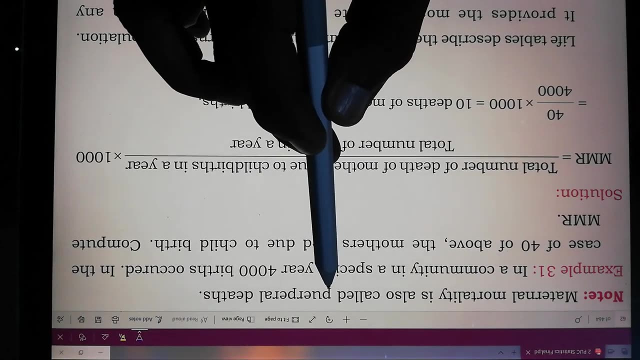 will come to know what you need to find out. I hope you understood. okay, right? neonatal mortality rate. we don't have any formal problems here. okay, let's solve maternity mortality rate. maternity mortality rate- maternal mortality rate. you remember this? it's also called as puperal deaths, puperal deaths- okay, right, see the formula problem in a. 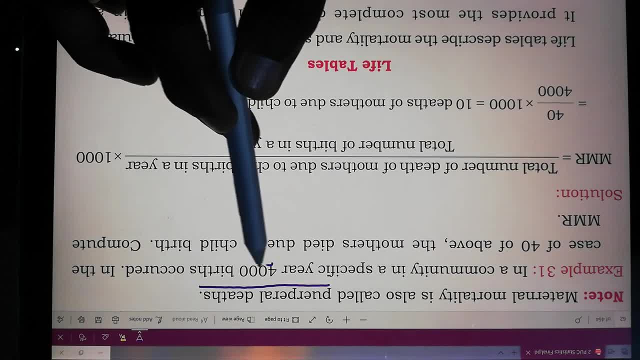 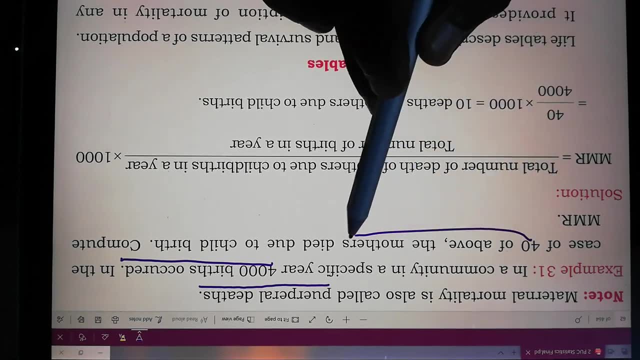 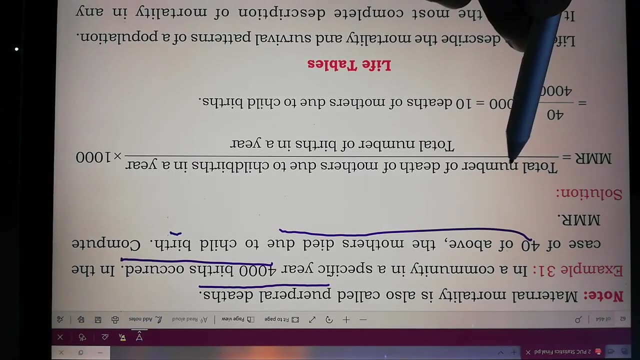 community. in a specific year, 4,000 births occurred. in the case of forty of the above, the mothers died. that means forty mothers died due to childbirth. okay, compute MMR. so what is the formula for MMR? total number of death of mothers due to childbirth in a year divided by total number of births in a year, into thousand. okay. 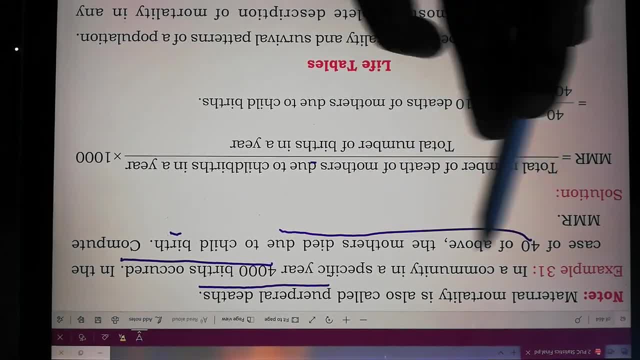 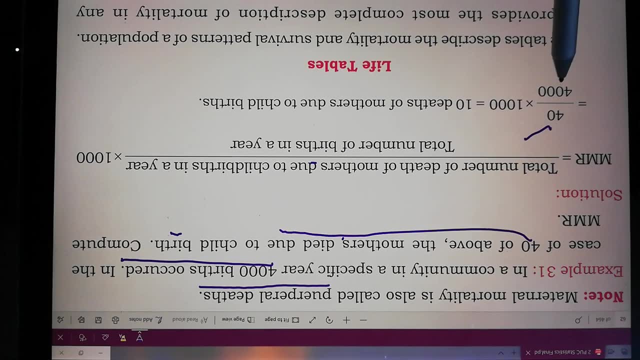 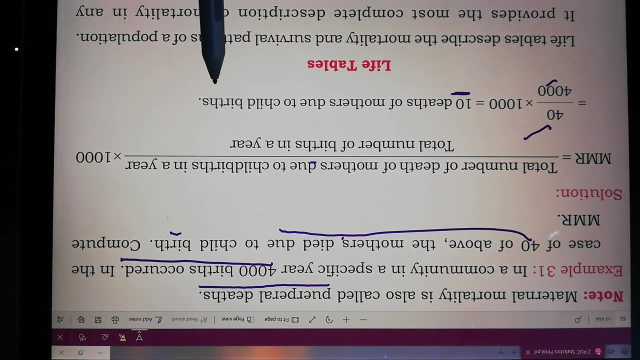 so how many deaths of mothers you see in this problem, 40 mothers died, so 40. you write, okay, total number of births in a year. how many 4000 births occur. that is 4000 into 1000. okay, you calculate how many. what is the answer? 10 deaths of mothers due to childbirths. this is the rate. 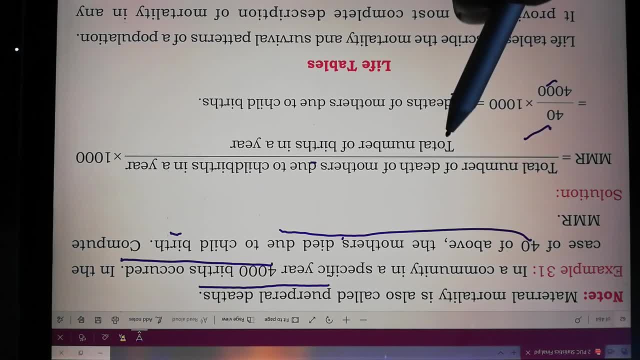 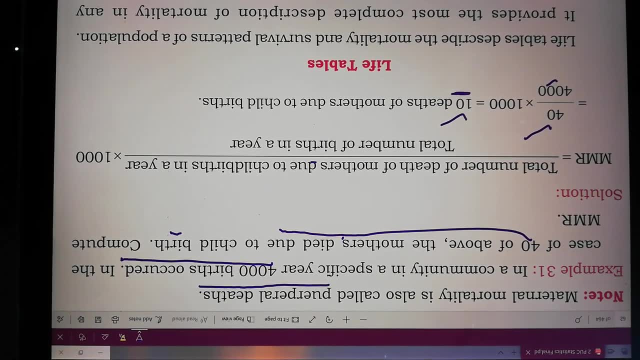 okay, the rate of maternal maternal mortality rate is 10. that means 10 mothers die due to childbirth for every thousand group of people. so this is what you can calculate, this mmr. okay. so we'll take some problems here. students, i will take some problems from the textbook. 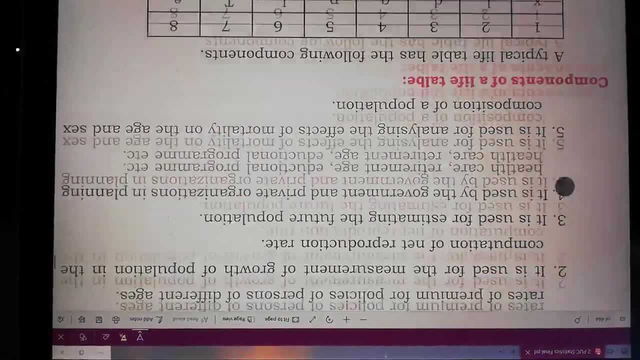 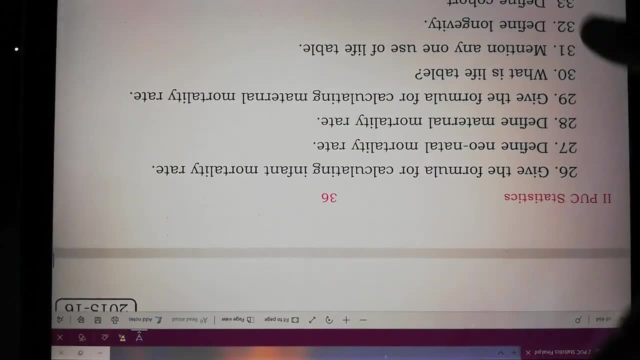 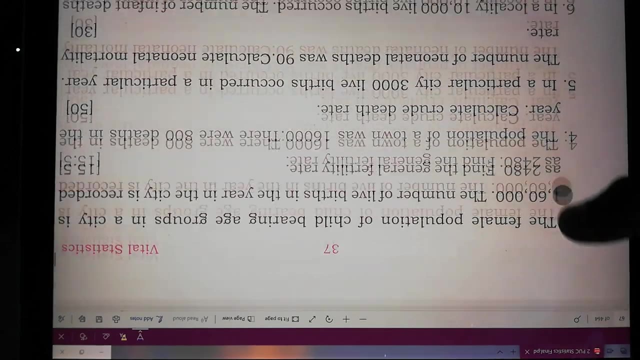 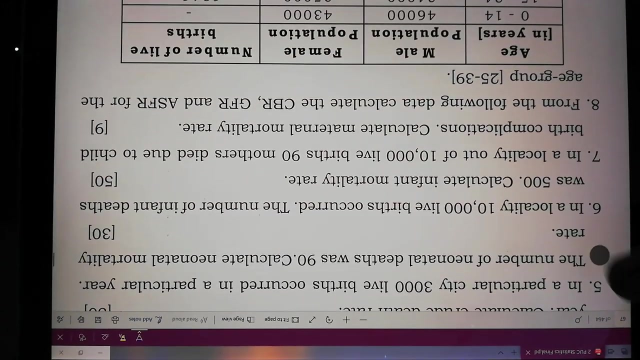 unsolved textbooks and then we will see how we can go about. okay right, let's take a two marks problems that we have it here and then we can go and solve some more problems. okay, later on with other rates. okay right, take the first ones here. calculate neonatal motor: fifth problem. fifth: 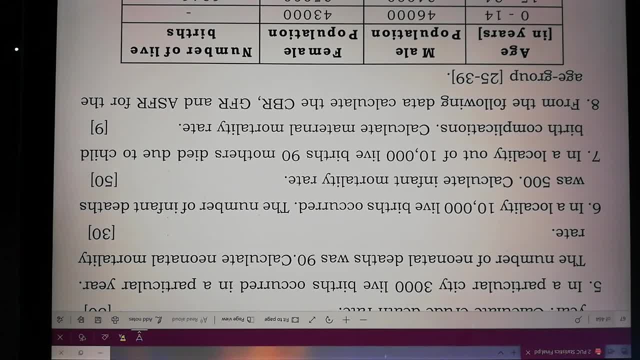 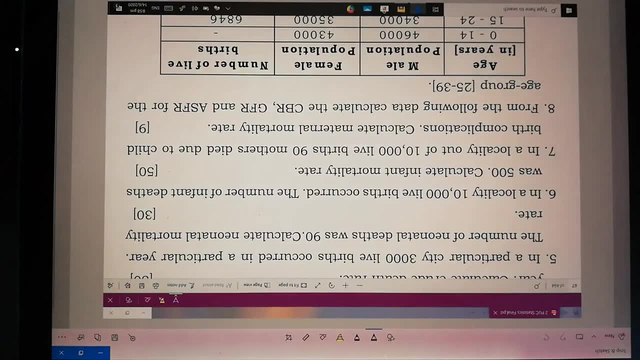 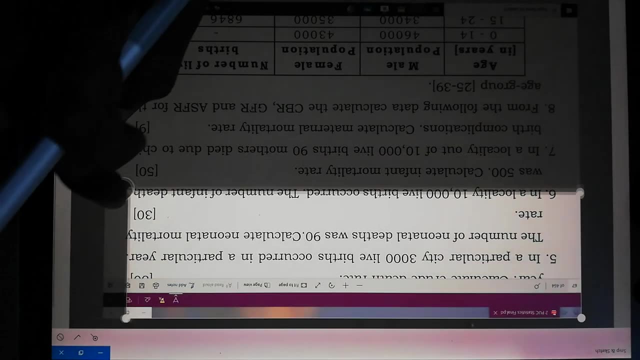 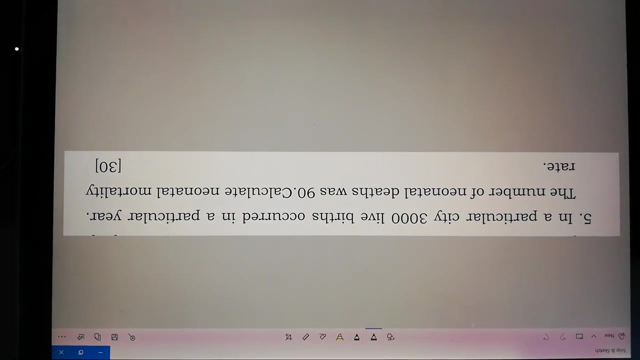 problem. okay, the fifth problem: in a particular city, 3,000 live births occur, okay, so I'll just crop it down, that question for you, so that it will be easy for you to understand and we can solve the problem in a in a nice way. okay, done, okay, see this: in a particular city, 3,000 alive births occurred in a. 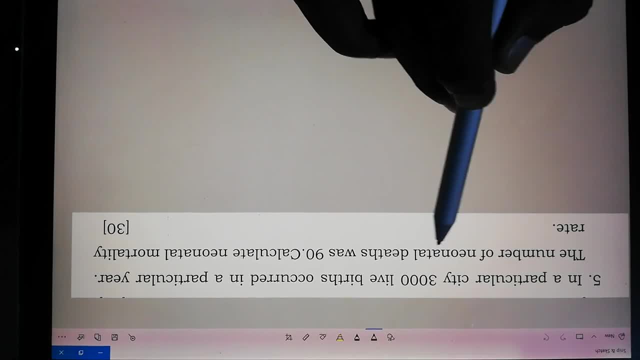 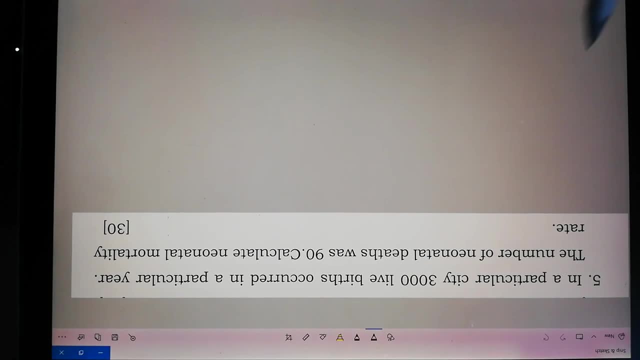 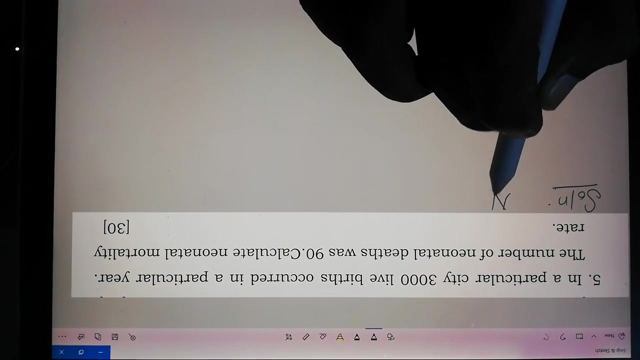 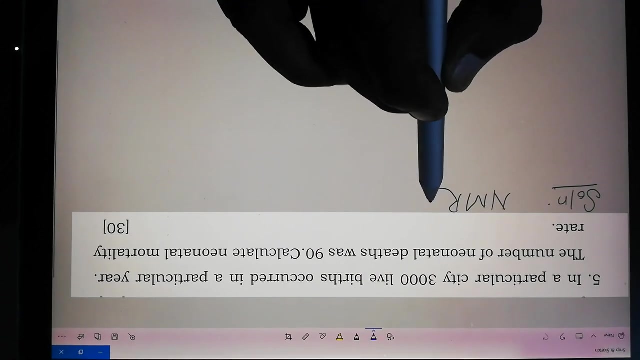 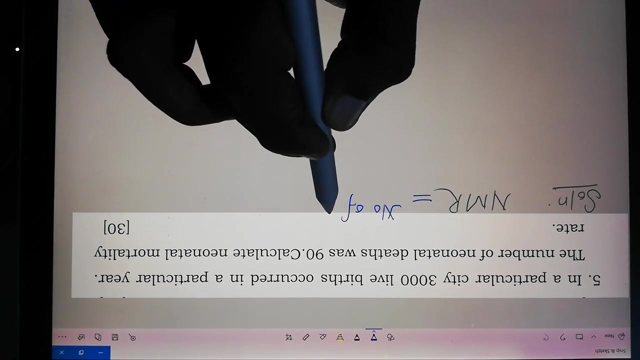 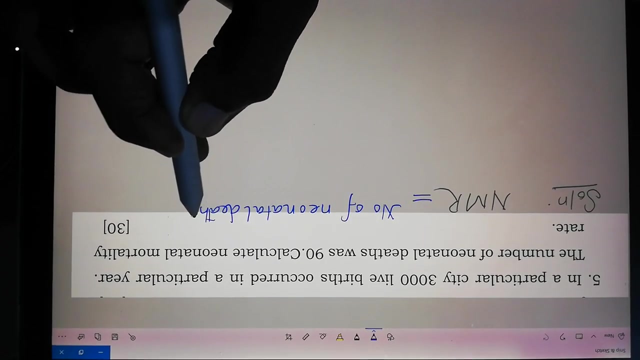 particular year, the number of neonatal deaths was 90. calculate neonatal mortality rate. okayanza workingghan. the first thing that we need to write down here is the formula for NNR. what is the formula for interest are okay, the formula for an MMR. what is a formula for an NR? the number of neonatal deaths in a year. Zero neonatal deaths in a year. Zero neonatal deaths in a year. 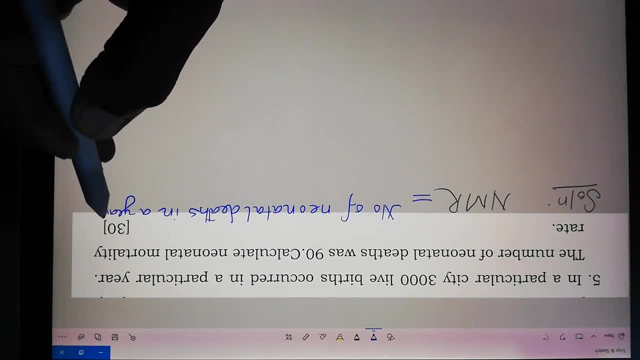 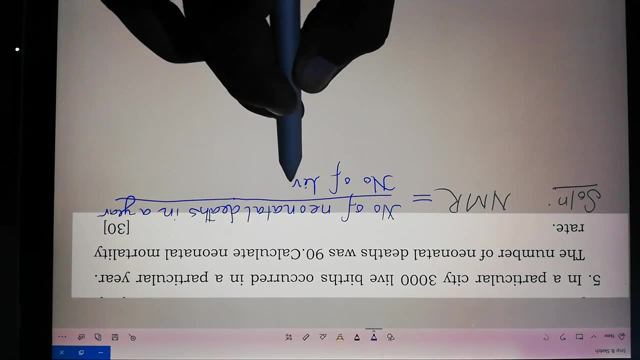 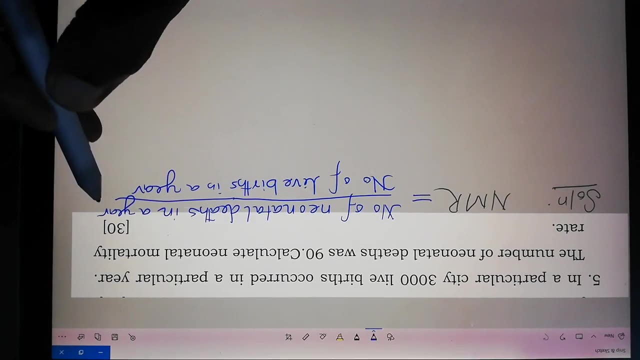 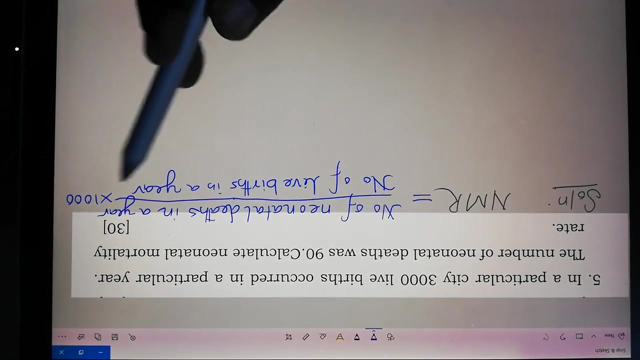 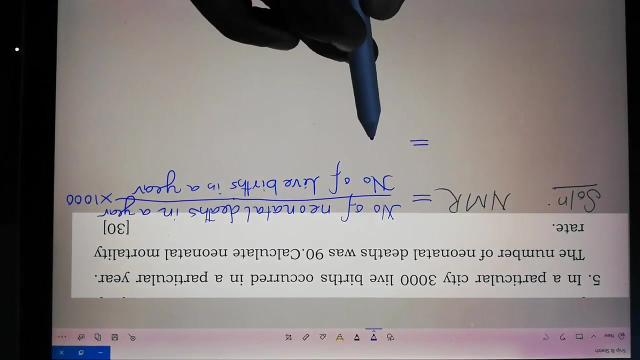 in a year divided by number of live births in a year in a year into thousand. correct: number of neonatal deaths in a year divided by number of live births in a year into thousand. so number of neonatal deaths in this problem is, in a particular city, three thousand live births. okay, number of live births is. 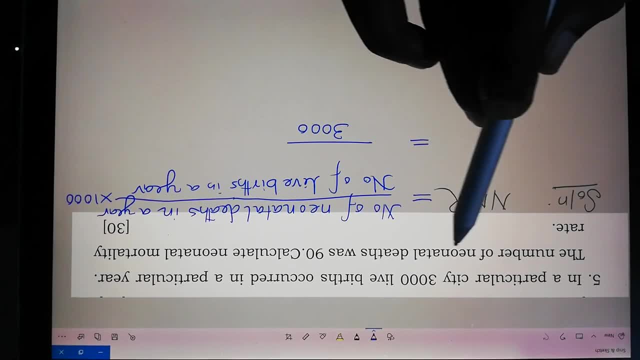 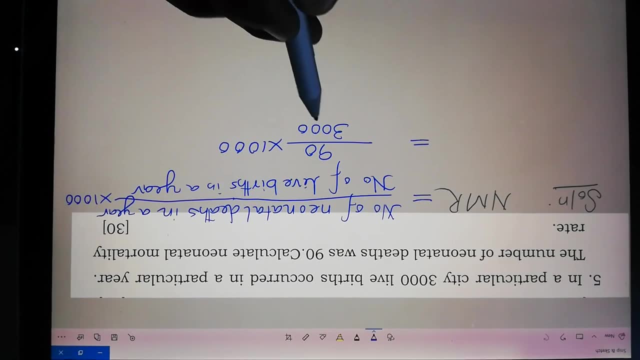 three thousand. the number of neonatal deaths is 90 into thousand. okay, so this three zeros gets cancels with this. three ones are three, thirties are. so the answer is 30. NMR is 30 deaths per thousand individuals per thousand live births in a year. 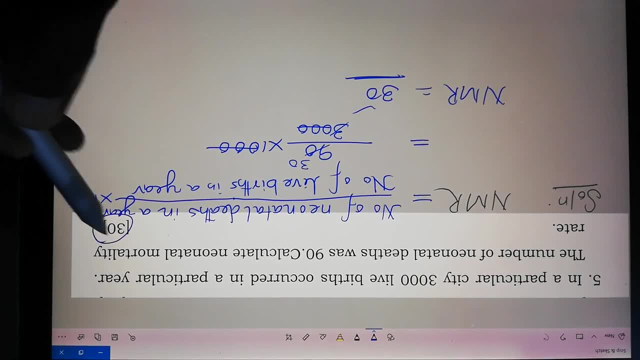 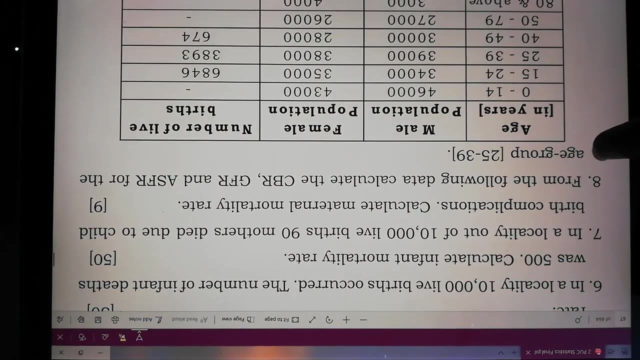 we get 30 neonatal deaths. so this is the answers here. is that okay? this is how we calculate a student's NMR. now the next one, if you just go for the next problem, right: infant mortality rates here. infant mortality rate: what is given to us? 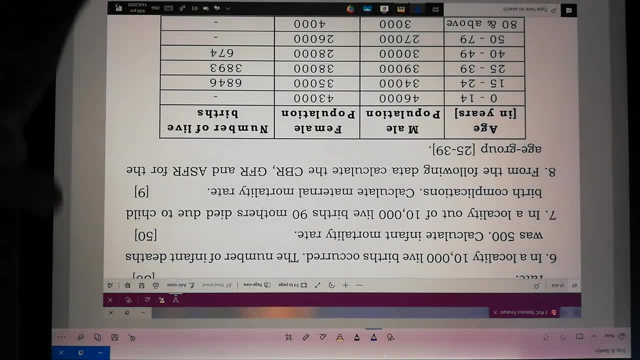 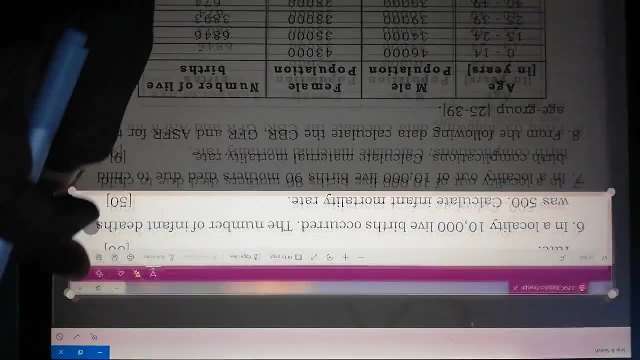 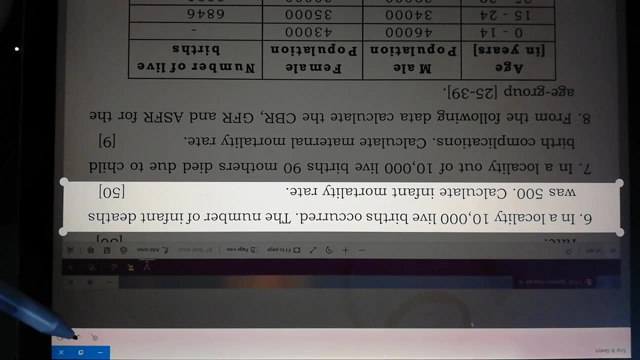 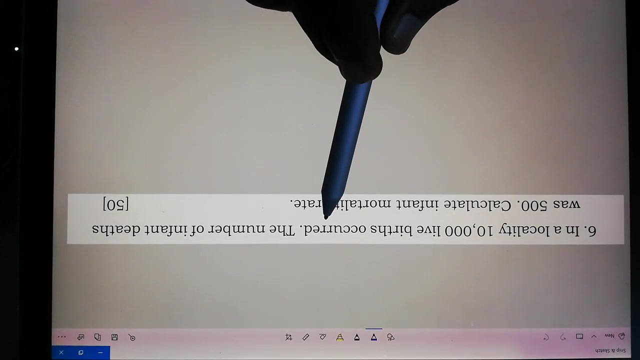 infant mortality rate. I'll just again crop this problem also for you. okay, let's see how we can solve this problem. and you, I have showed it to you once again, let's see how we can do it. okay, see you. in a locality, ten thousand live births occurred. in a locality, 10,000 life births occur. the number of infant. 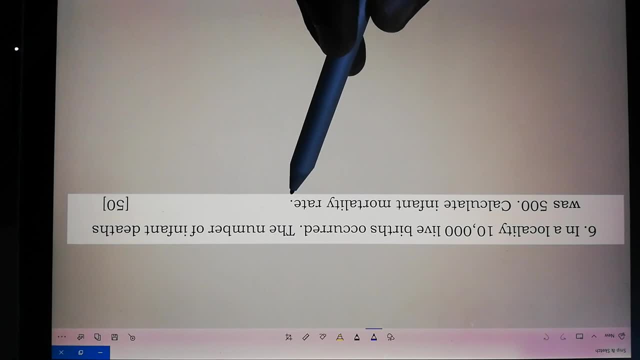 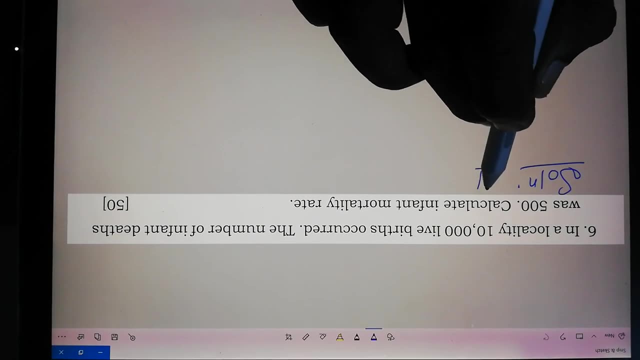 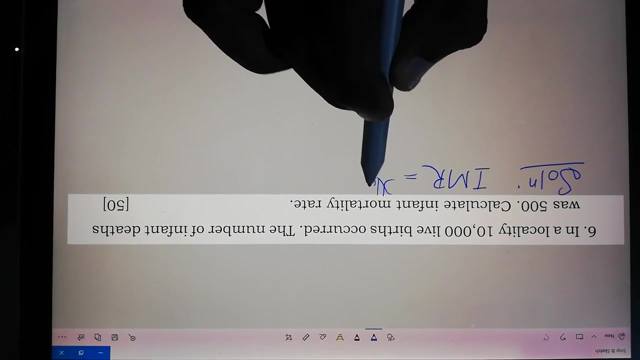 deaths was 500. calculate infant mortality rate. so for us, the first thing that we need to write, as I said, is which care is based upon results under this one mark is the formula IMR. IMR is equal to number of infant deaths. number of infant deaths. 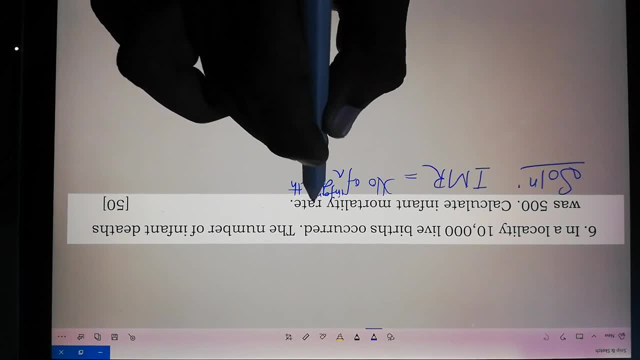 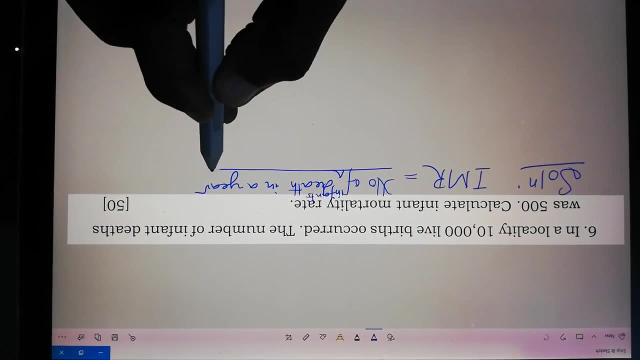 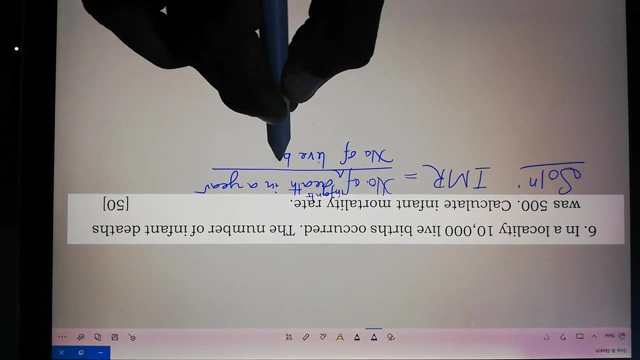 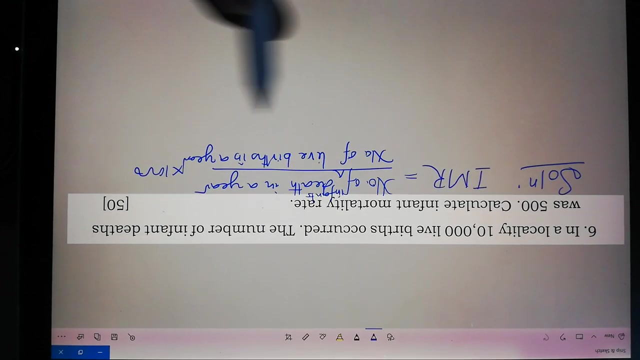 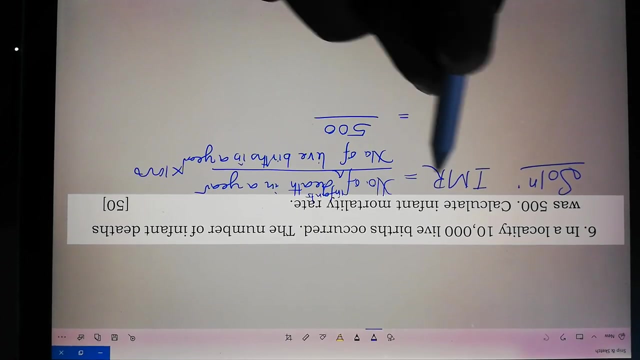 or number of death of infants. infant deaths in a year divided by number of life births. number of life births in a year into thousand: okay, So number of infant deaths, number of infant deaths, is 500, 500, in a locality, 10,000 life births occurred. 10,000 life births. 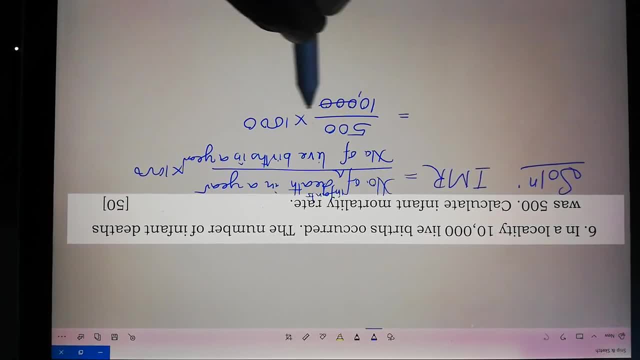 occurred into thousand, This one, these three zeros, and these three zeros cancels, okay, Cancels. What is the answer? 50. That means infants, 50 infants per thousand life births die. This is the simple calculation. IMR is equal to 50.. See, you got the answer. it's. 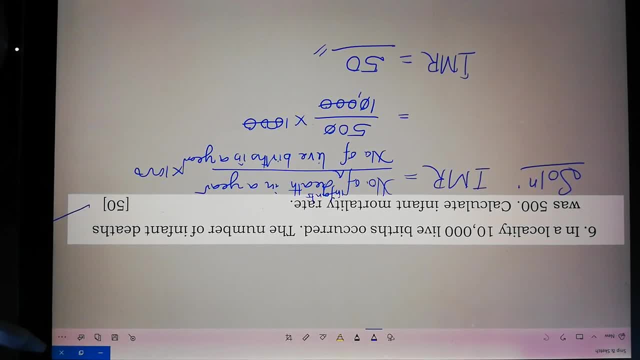 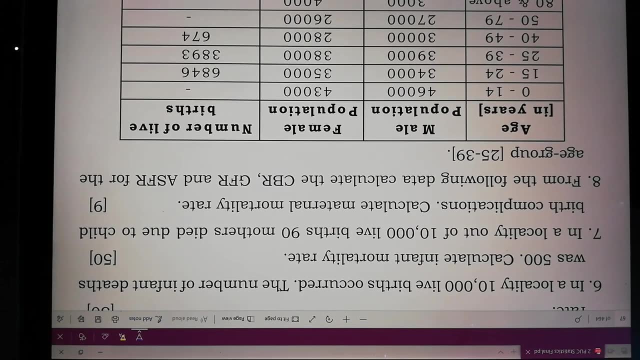 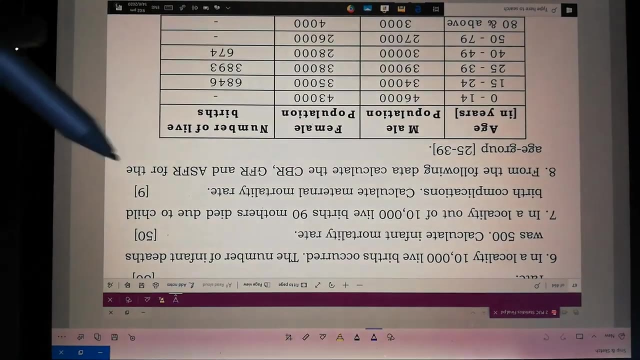 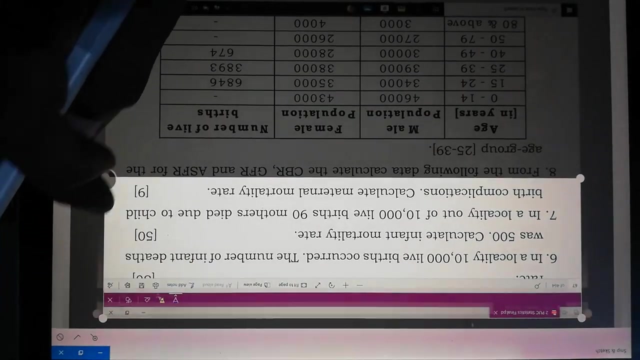 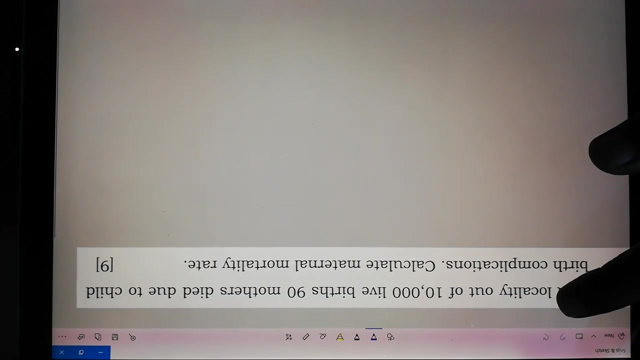 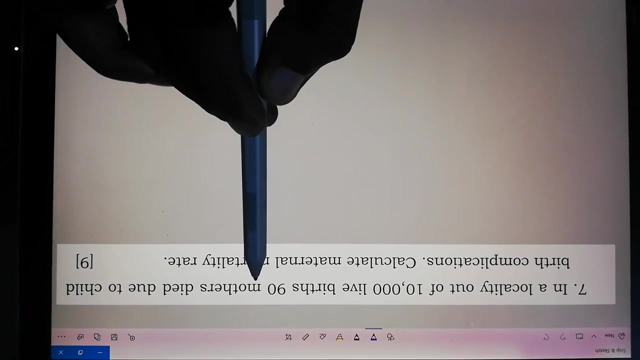 50,. okay, Right, we'll take the next one. Next one is calculate maternal mortality, Maternal mortality rate. okay, This also will. I'll crop it for you. okay, Only, let's take this right. In a locality, out of 10,000 life births, 90 mothers died due to child. 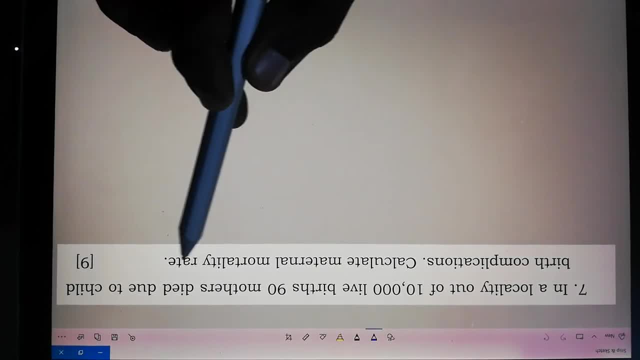 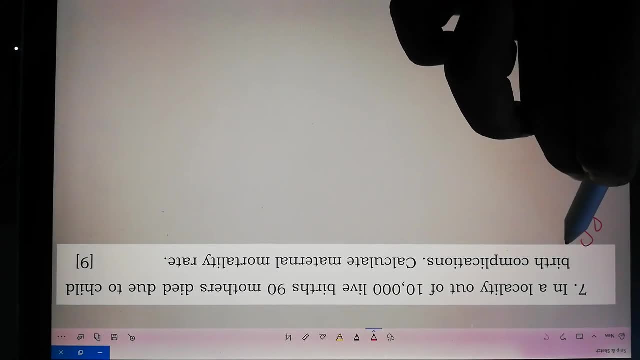 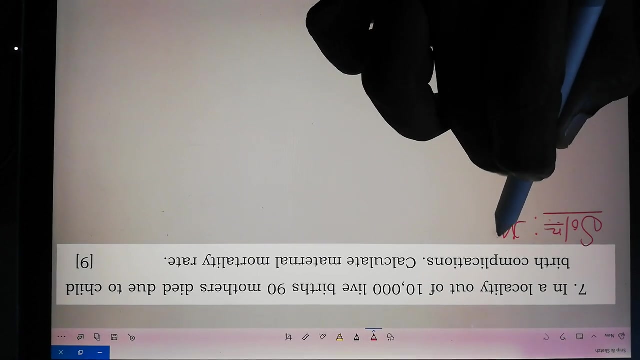 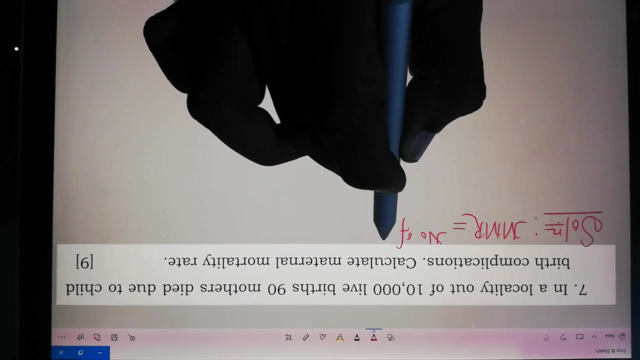 births. Child birth complications. Calculate maternal mortality rate. okay, Calculate maternal mortality rate. So the first thing, that, again, what you need to do is to write the formula, The formula for MMR maternal mortality rate. What is that formula? That is number of number. 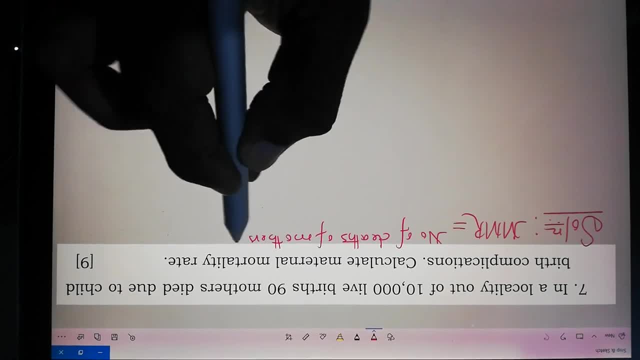 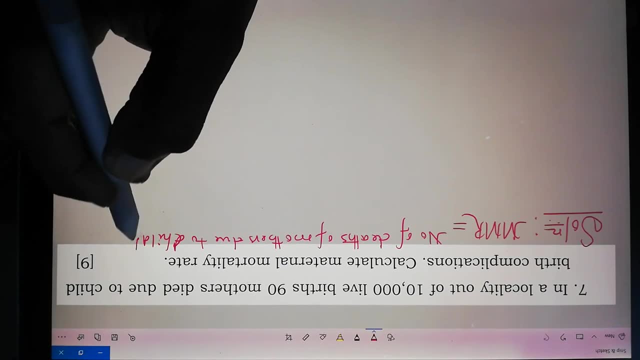 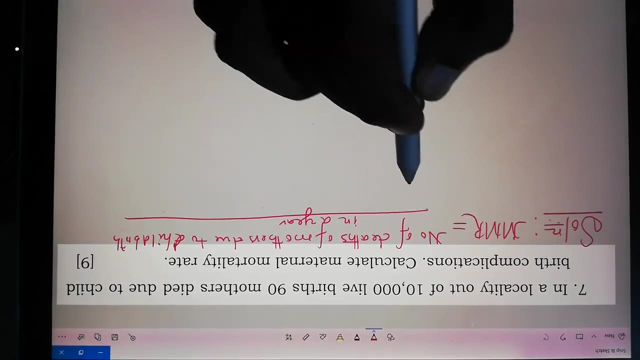 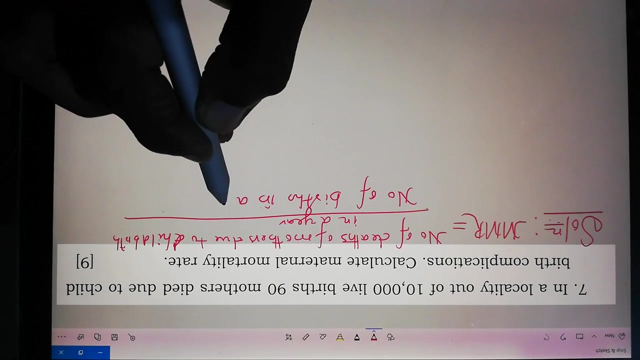 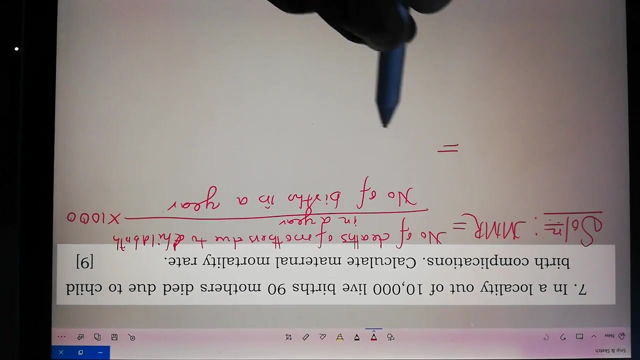 of deaths of mothers: number of deaths of mothers due to child birth- due to child birth in a year, divided by number of births in a year, into thousand. okay, So that's the formula. Okay, So now see number of deaths of mothers in a locality out of 10,000 live births: okay, 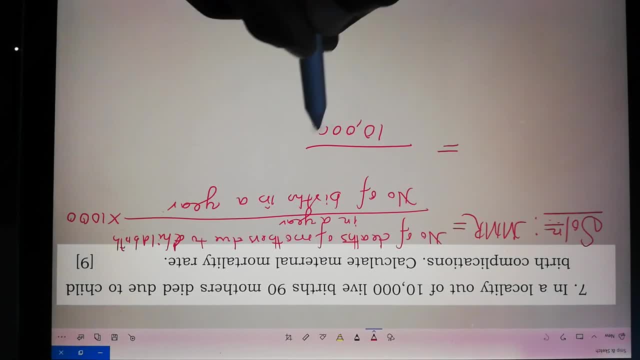 This is 10,000 live births, 90 mothers died, 90 mothers died in 2000,. okay, So these three, these three gets cancelled, This zero, this zero gets cancelled. The answer is nine. So nine mothers die per. 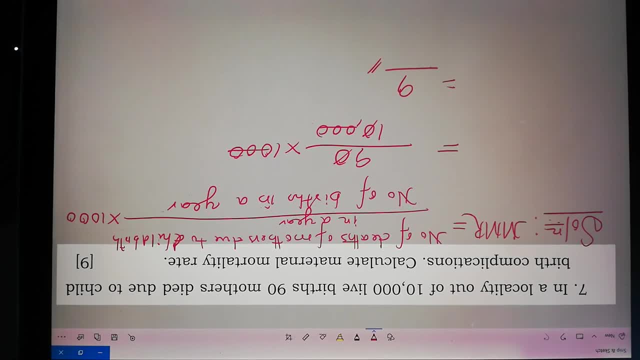 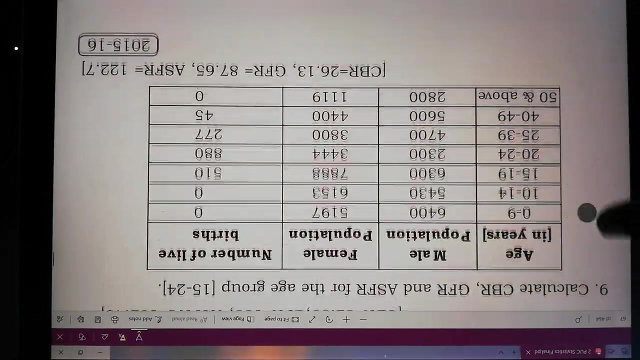 thousand live births. nine mothers die per thousand live births. so the answer is nine, so we got it nine. so this is how we solve these problems of imr, nmr and mmr: even if they give certain type of a data. let's see if we have any type such kind of a problems where data is given. 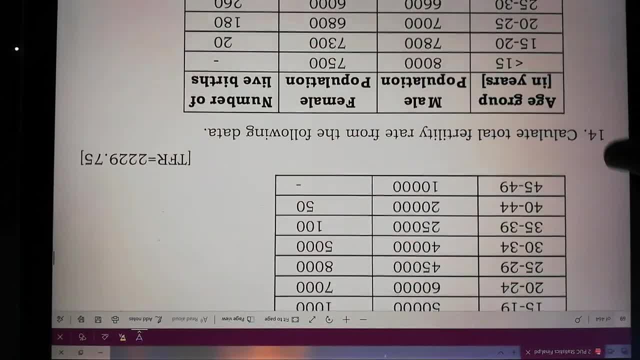 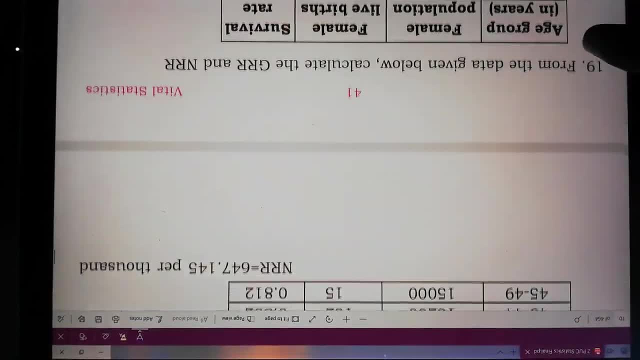 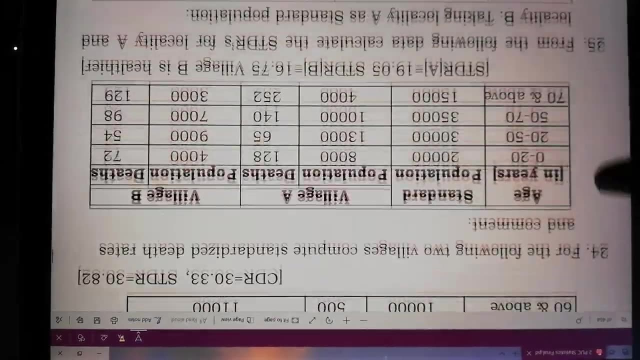 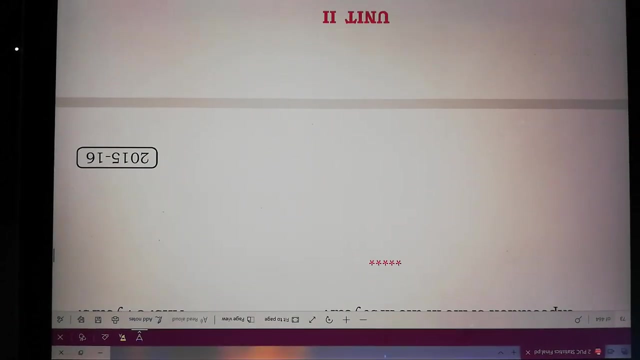 with all the age, age group and all. let's see if ever we have to solve the problems for that. also, if it is not given, then it's okay, because not important for us to solve those problems of that type, because this we need to always practice. students from this textbook on the 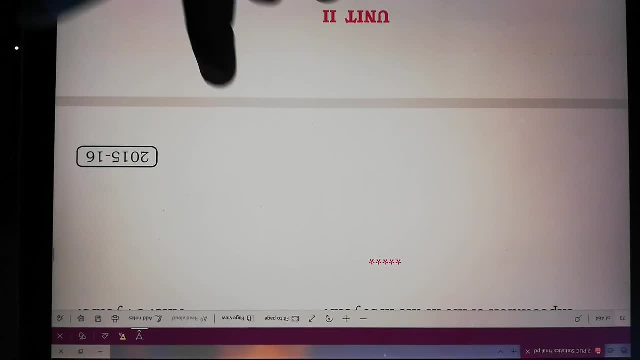 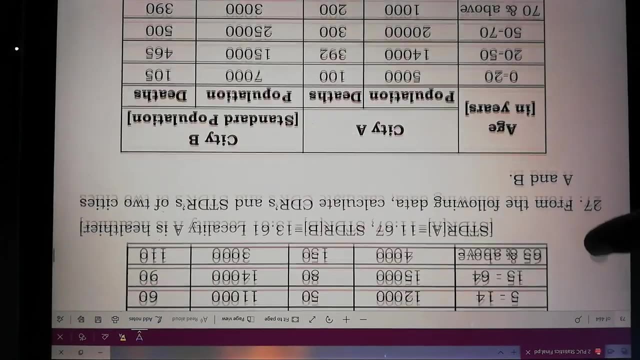 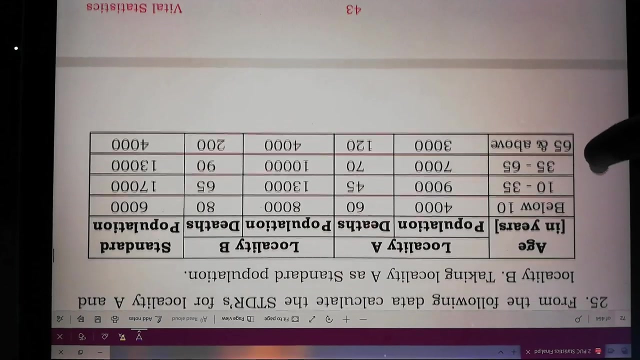 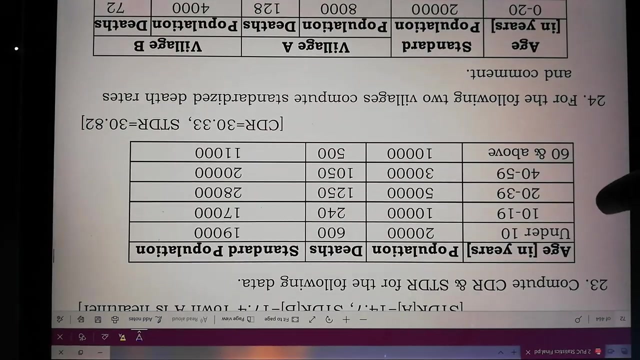 maximum is from the textbook itself. so see that you are always following a textbook students, this textbook itself. so whatever problems are there, that is the reason why i have taken all the problems from the textbook, solved problems from the textbook and i'm giving assignments also from the government prescribed assignment panel those 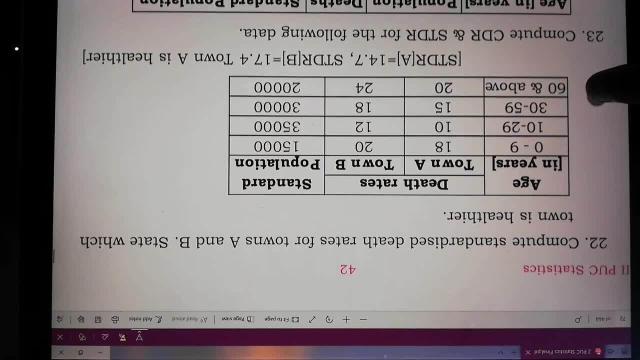 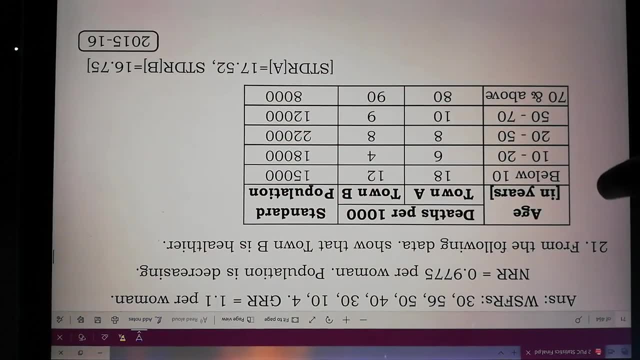 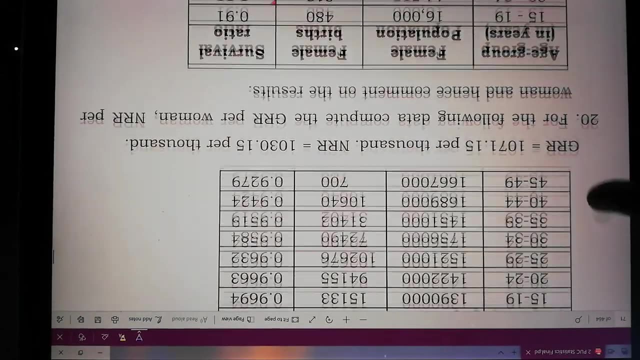 people have released those assignments for us, so we have. i'm giving the assignments from there itself, so do not neglect them. please do solve them. it will be very much helpful for you. okay, so we don't have any problems based on this. uh, imr and and, imr, nmr and mmr right now, so whatever. 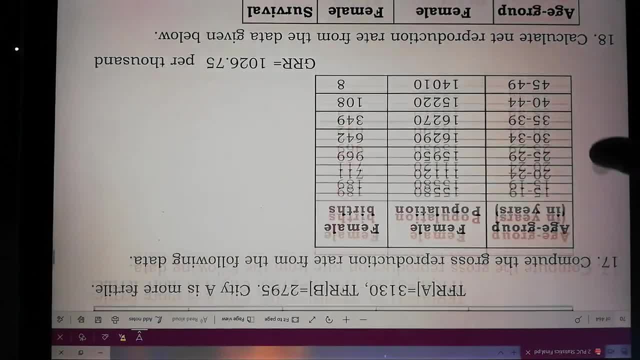 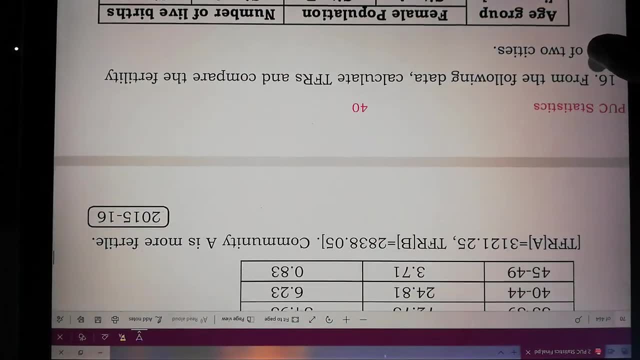 i have solved, whatever i have solved. only those are there. so we will end the class today here, right now. so in the next class we will solve the problems on stdr students. okay, stdr, okay, fine, thank you very much. 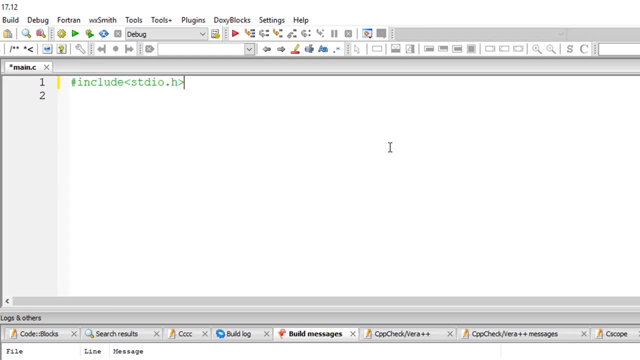 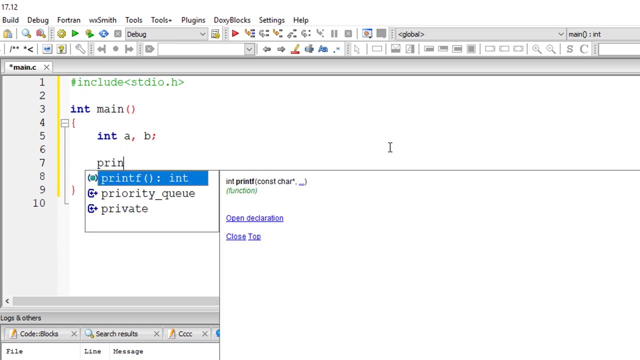 Let's see how we can add two numbers in C program. So I'll include stdioh and write int main int, because our main function returns an integer value, So I'll return zero. I'll take two integer variables, a and b. I'll ask the user to input values for a as well as b using scanf. 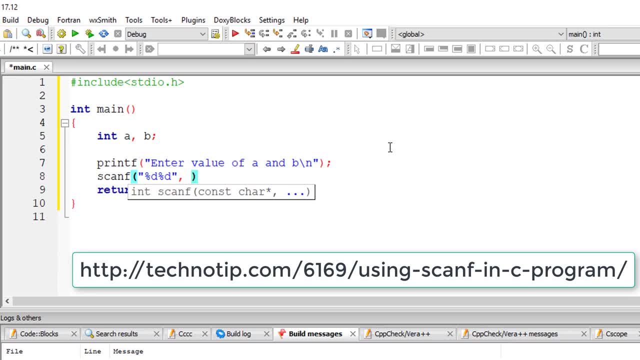 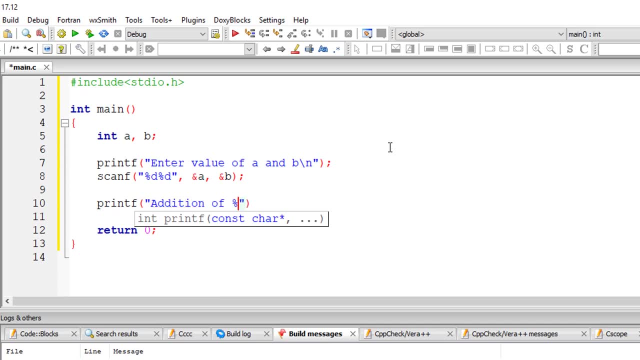 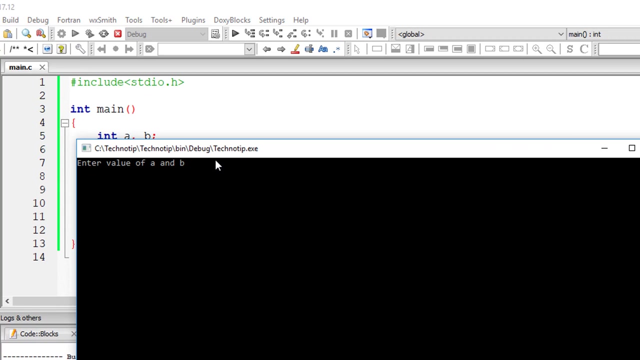 I'll store the values in ampersand a and ampersand b. that is address of a and b. Now I'll output the addition of a plus b in printf statement itself. I'll write a plus b here. So that's it. This is how we can add two numbers in C. 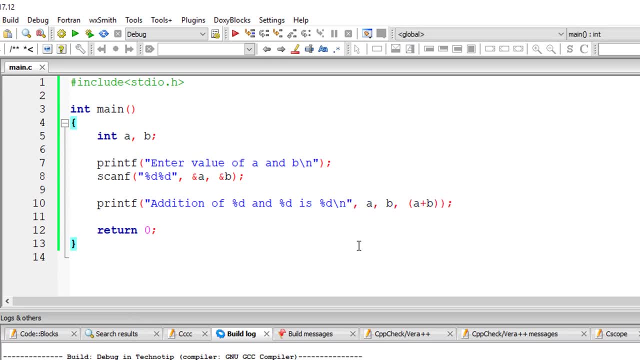 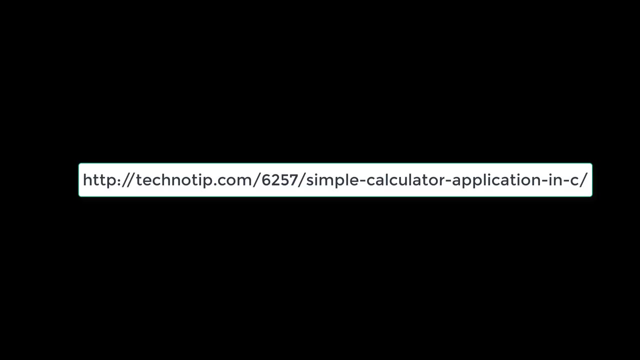 I'll add a new line character here. You can also take another variable c and then write expression here c is equal to a plus b and then replace this a plus b with variable c. So I'm writing this application as a building block for calculator application. So stay tuned.